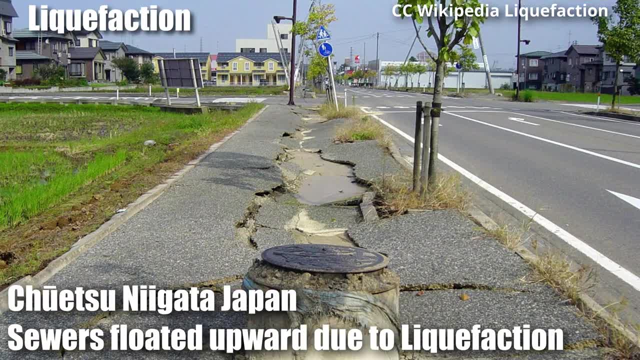 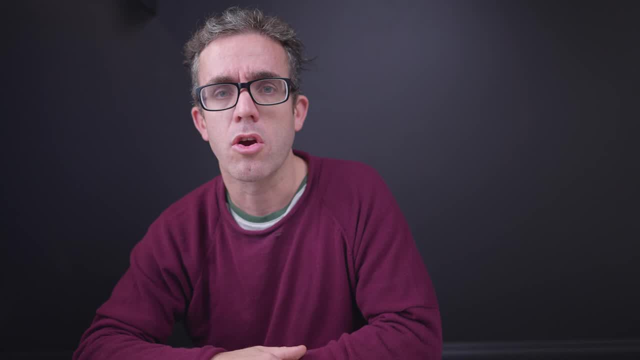 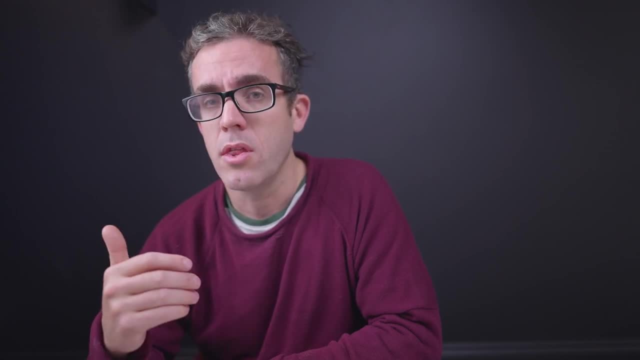 And this is liquefaction. Liquefaction is when the ground actions cause the soil to essentially act like a liquid, or liquefy, as the name suggests, So it's no longer going to be able to resist those vertical actions applied to it. These type of events can actually even be more damaging than the effects of what the earthquake would have had if it was just to shake the ground. 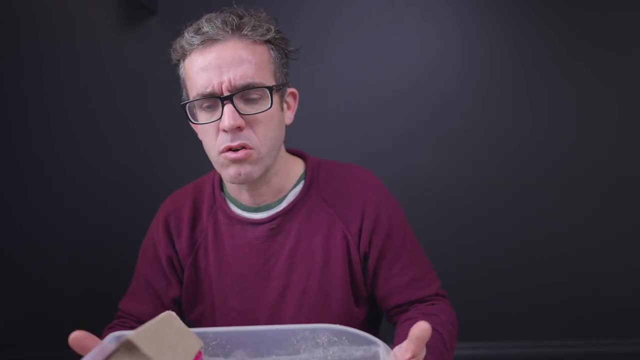 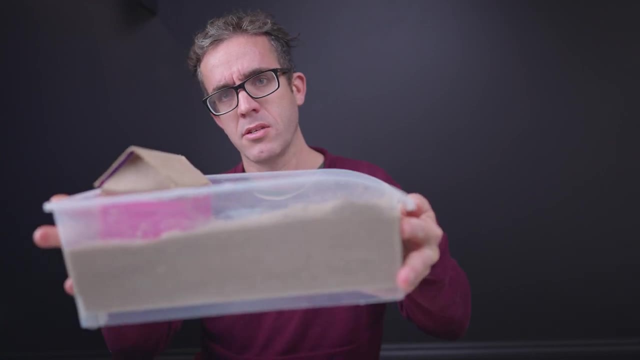 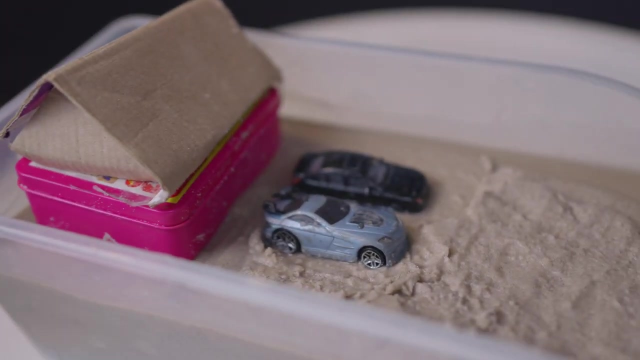 And the great thing about liquefaction? it leads to a great practical example that I'm going to present here today, And all we need is A box of sand, some props in here and a little bit of water. From this practical example, you're about to see what effects liquefaction could have on your structure and how you may need to design for them. 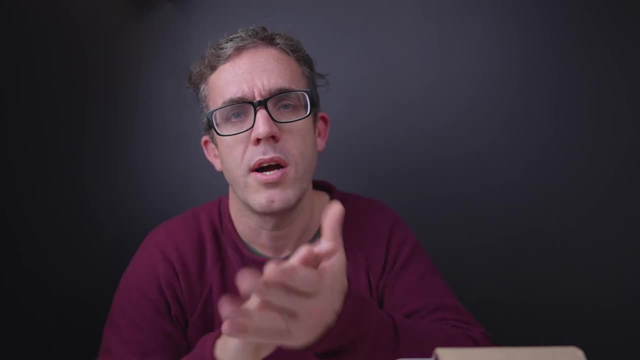 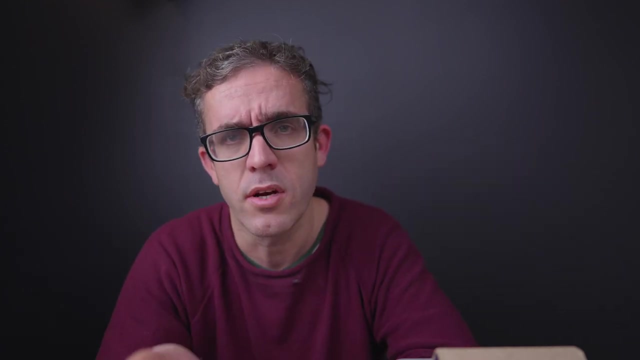 So the type of soils that can be affected from liquefaction require two things: You require a coarse-grained soil that allows water to seep in there, And you need that high water table to allow for the sprains to slide against each other. 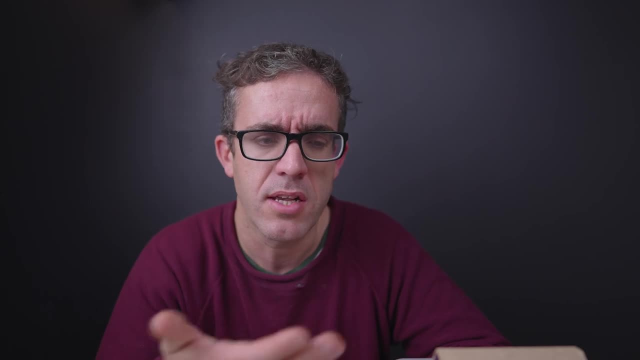 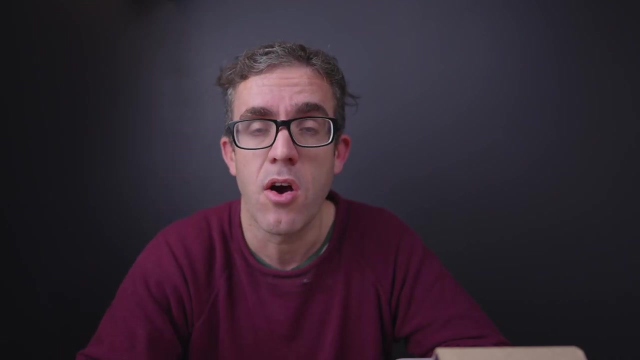 When the ground shakes, during an earthquake, what it does? It makes the ground more free. It also raises that water table as well. So not only do the structures sink in, lighter objects will actually rise to the surface, And from this demonstration you'll see that the soil will no longer be able to take any vertical or shear forces. 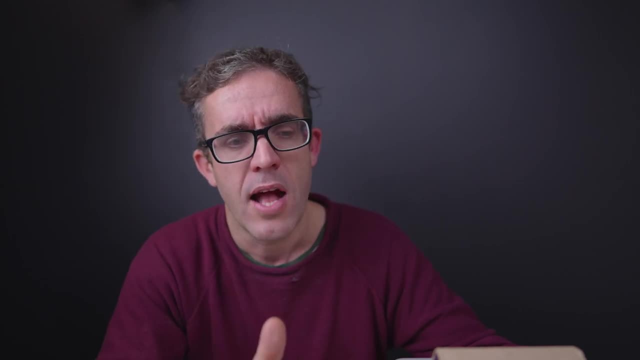 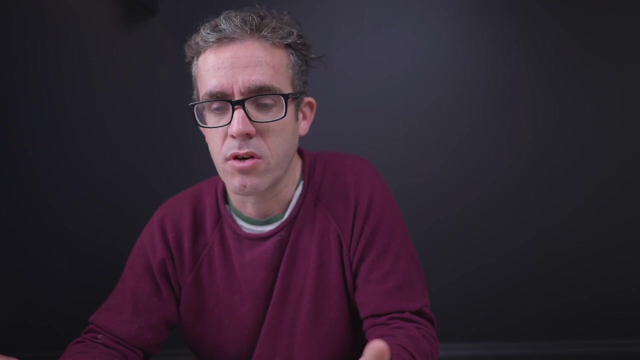 However, those shear forces will be highly dissipated, As the same actions that are allowing the structures to sink into the ground will no longer allow for those shear actions to be dissipated through the soil. So, with this practical example, It will give you a more clear understanding of what effects liquefaction can have on your structure. 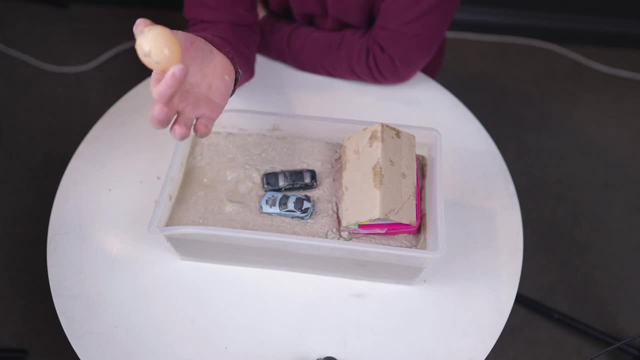 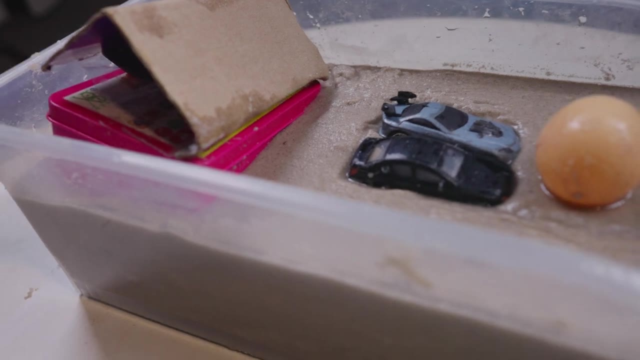 The soil was liquefying, So we had a really light object underneath the soil that has now risen to the surface. Meanwhile the other structures and cars have started to sink into the ground, But, as we saw when we were shaking, that water table was rising to the surface as well. 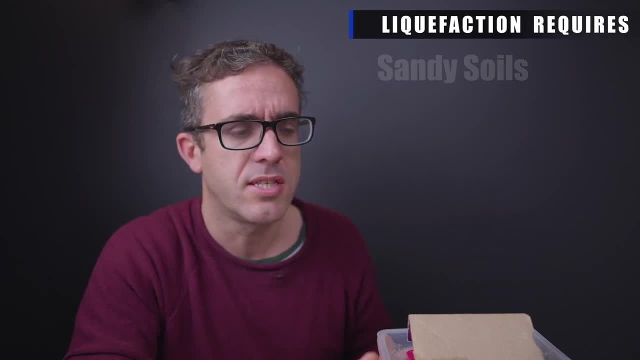 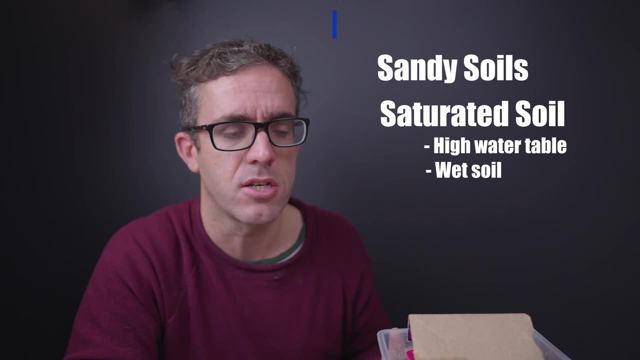 Liquefaction only occurs under unique circumstances, So in a sandy type soil with a high water table And also requiring that earthquake to allow for the soil to liquefy. under such an event, If you're enjoying this practical demonstration of liquefaction, Don't forget to liquefy the like button. 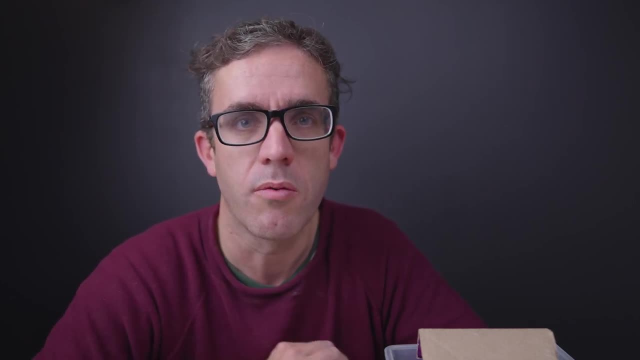 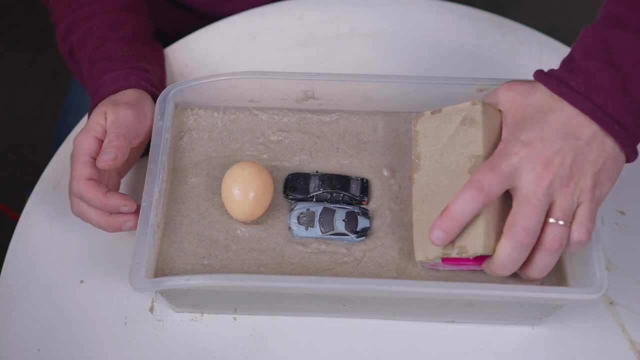 Not only does it help me out, but it encourages me to keep doing what I'm doing Now. let's keep going with this liquefaction event. So let's remove our structure and see how deep it's actually gone into the soil So we can see it's gone quite a long way. 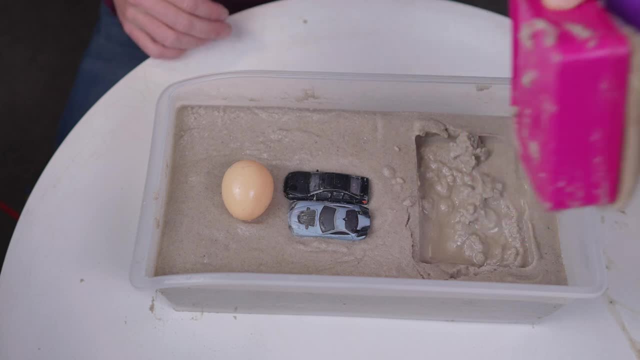 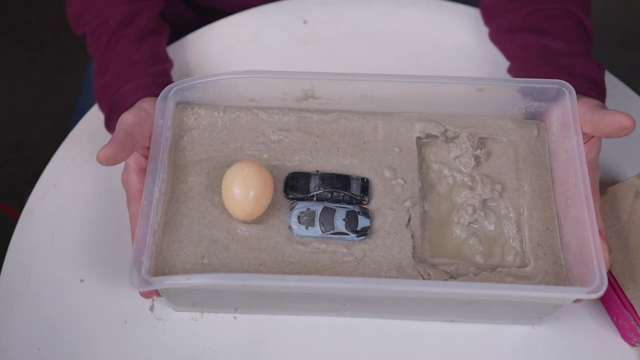 And you can see the water table has risen quite high here as well, So we're able to keep shaking it without the structure. actually there We are able to see that the soil is behaving more like a liquid than it is a solid. As I reintegrate. 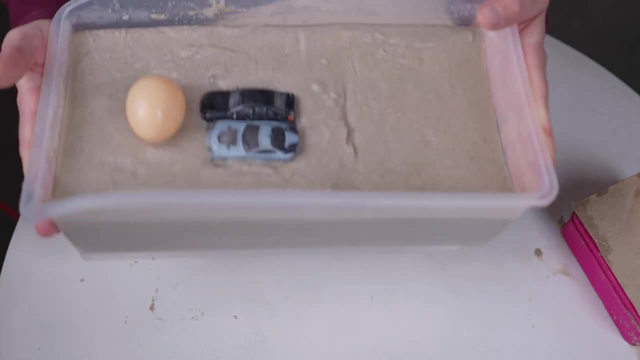 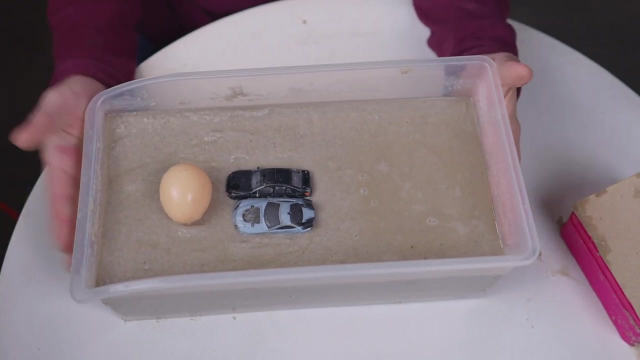 Essentially making the hole non-existent, with the structure no longer there, And even from that, you can see how it's rocking backwards and forwards and behaving more like a liquid From the shaking actions that have been applied to it. So how can we resist it? 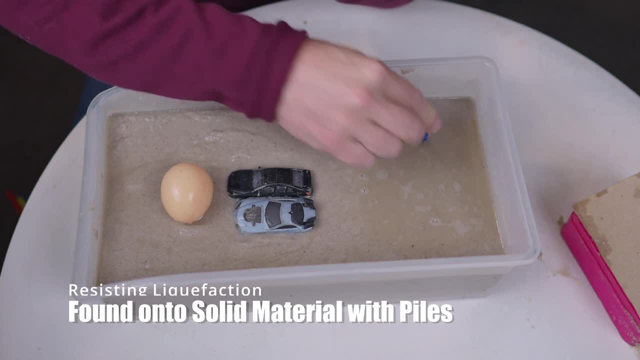 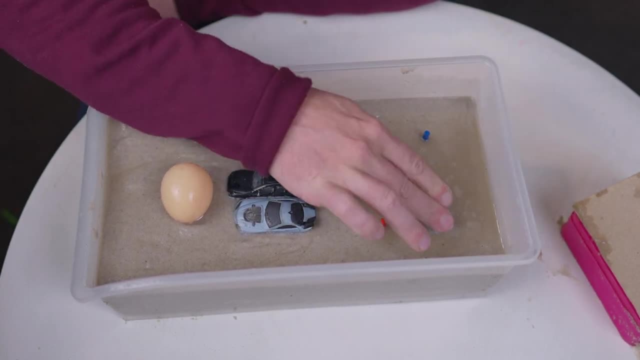 This is simple really, And that's through putting a series of piles down Down to a solid founding material. I'm not sure if you can see what the problem is going to be. See if you can guess before I actually put the structure down. 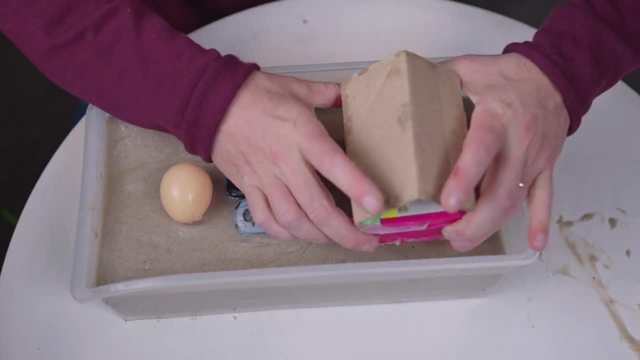 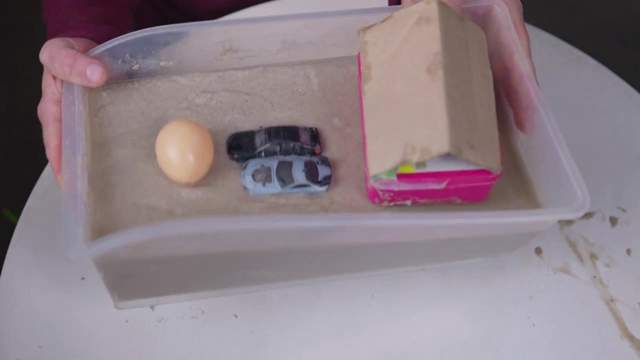 What issues we might have from these piles being able to keep the structure upright. See the structure So we can push down on it. It's solid, But now let's shake it and see what happens While the structure is still standing up. 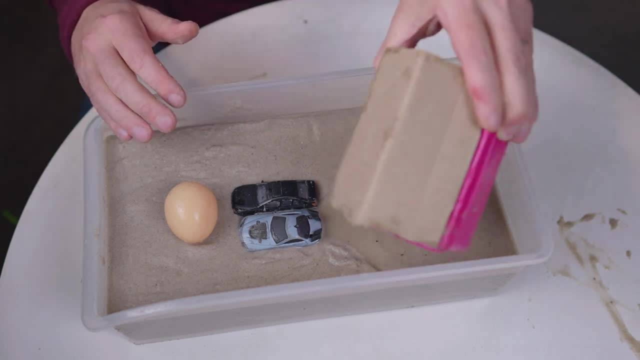 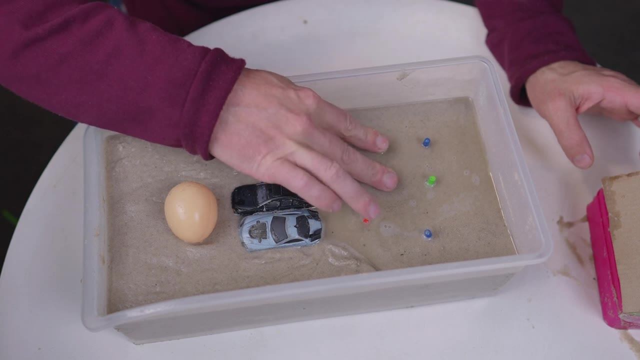 It's rotated off it's axis And if we have a look at the piles underneath, We can see that they are now not necessarily all of them upright. We've got these ones here. They can still take resisting forces. And we've got these other ones now. 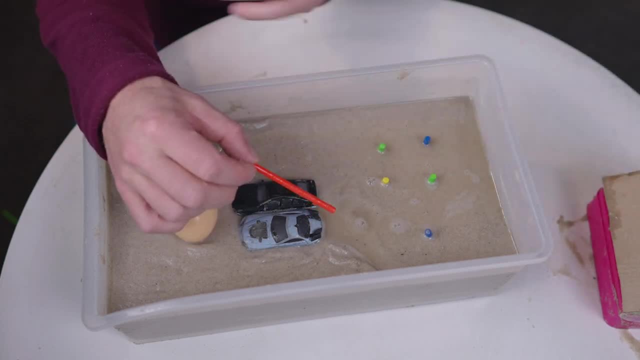 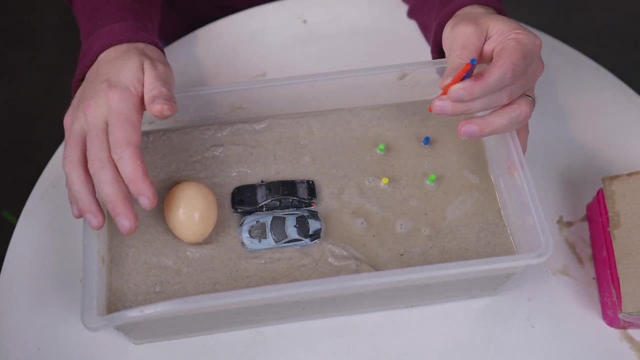 Where the structure has shifted sideways from the lateral forces And now, As the soil is no longer able to resist those shear actions That the piles are applying to it. So those piles, Although they're founded back onto the bedrock, Yes, they can resist the vertical forces. 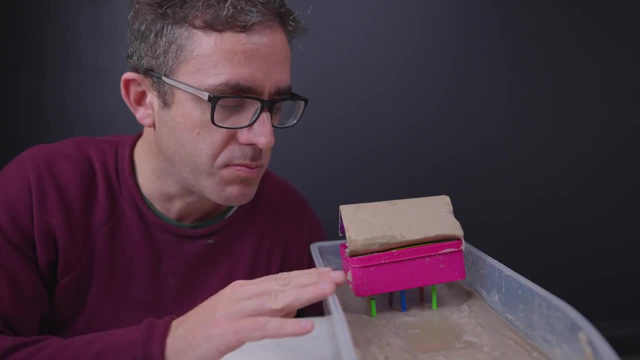 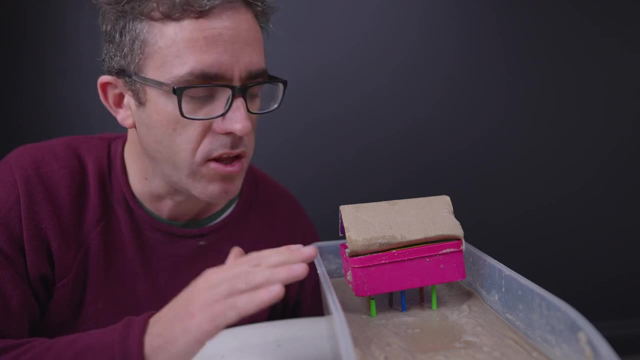 But they don't have the soil there to resist those lateral actions. So we can see from this building where we've got the building above ground. We would see that the piles would need to resist those lateral forces. Now a similar thing has happened during the liquefaction event. 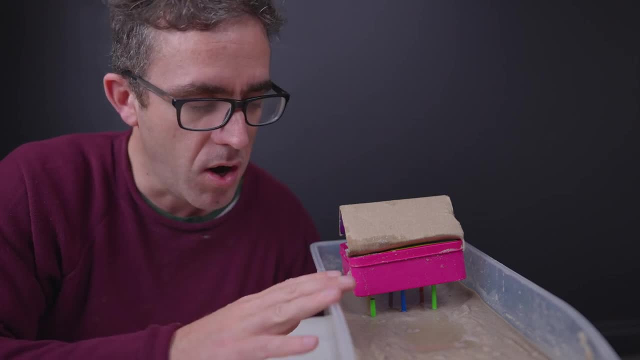 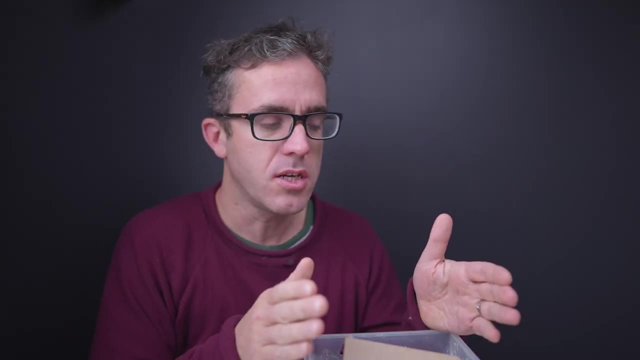 So the soil is no longer to resist any of those shear actions. So the piles need to have some way of stabilizing themselves From the more solid bedrock. There's a number of ways we can deal with this. We can obviously design the piles to cantilever off the bedrock.